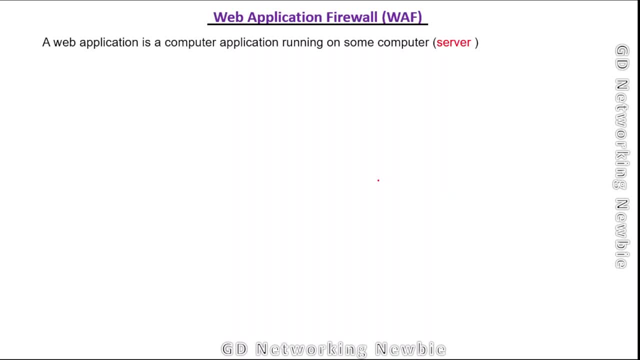 Hi everyone. today we are going to discuss about WEF. So WEF stands for Web Application Firewall. So first of all let's see what web applications are. So web application is a computer program or application software running on some specific computer. So let's say we call that computer a. 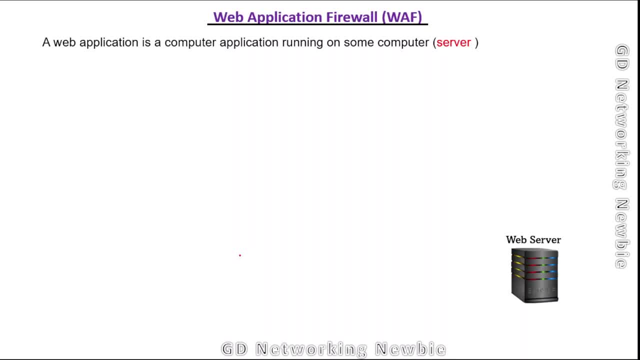 server. Let's say we have this server and on this server we can have different kind of web application, like banking application, student management system or ERP. or let's say we can have a gmail, simply. So let's say gmail is a web application and now to access that gmail we use. 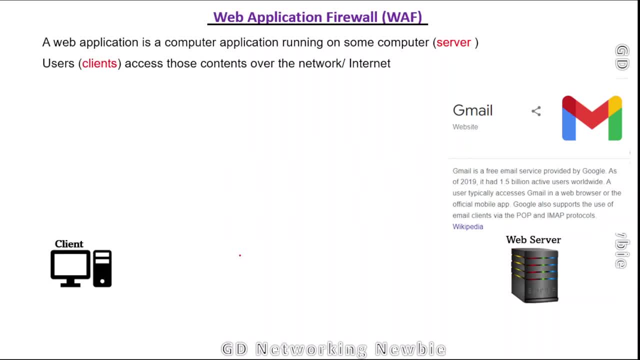 our computers. That computer can be laptop, smartphone, tablet, and we call that computer a client machine. and on that client machine we open a web browser and using that web browser and using some network or internet connection, we can access those web applications, which may be hosted in any other corner of the world. 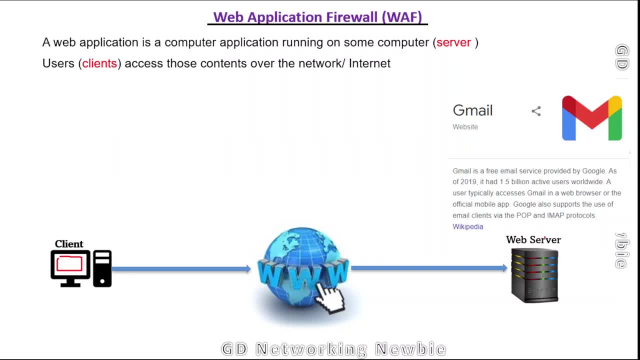 And now, let's say, in these web applications, which are again some group of instructions at this computer program and in that computer program, we can have some weaknesses, And those weaknesses or the vulnerabilities can be exploited by this bad guy using the same network or internet connection. They may find some weaknesses here and then, using those weaknesses, they can exploit. 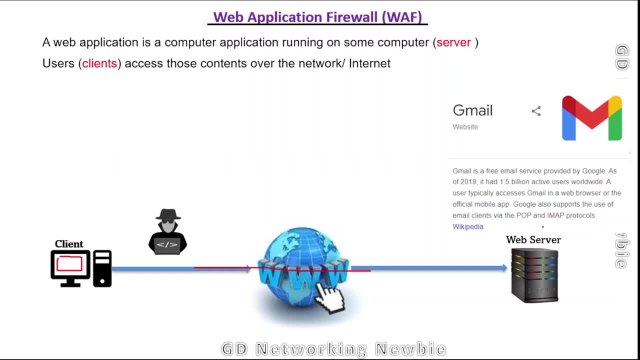 our system. So now we'll talk a bit about the equipment being one of the main uses. where can we have moment- agents and announcement? so this is an interest that we will talk about in this lecture, and then we'll talk about how to fix, for example, to fix an. 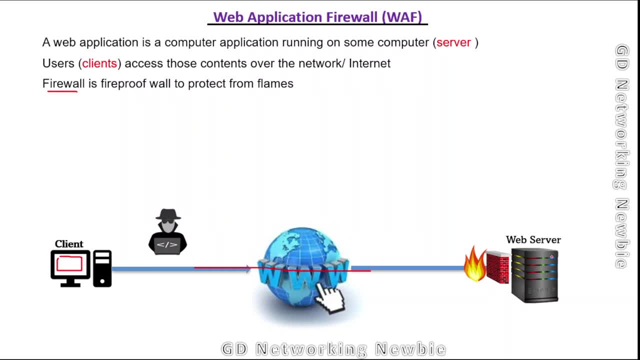 offender. If we olhar this far, so you can see that my left hand is motivated by a control panel part and right hand is controlled by the only other control panel on this app. And this is the control panel process, and which means the server has the payments too. 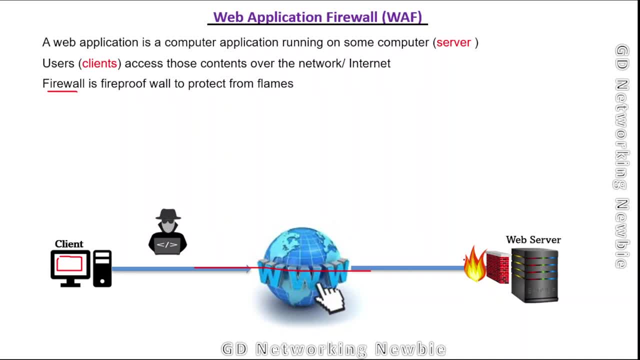 And when you come into this site, like I just came into this site, there is no such command in our or our web application from these flames. so this flames here means there is some malicious traffic or some malicious packet with bad intention they want to cross or they want to reach. 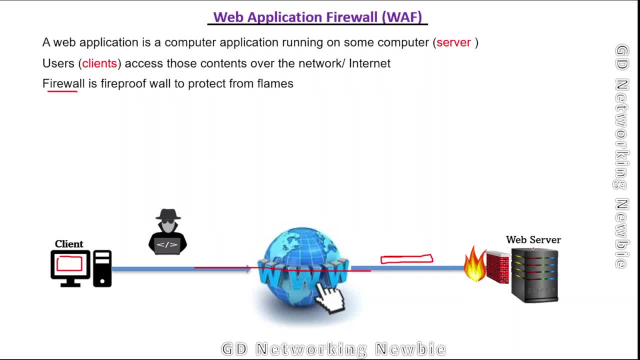 at our web application, to exploit it or to destroy it. let's say so now. these web applications needs to be protected, and for that we have this firewall. and now for this firewall, let's say draw it again here. so for this firewall to decide or to protect. 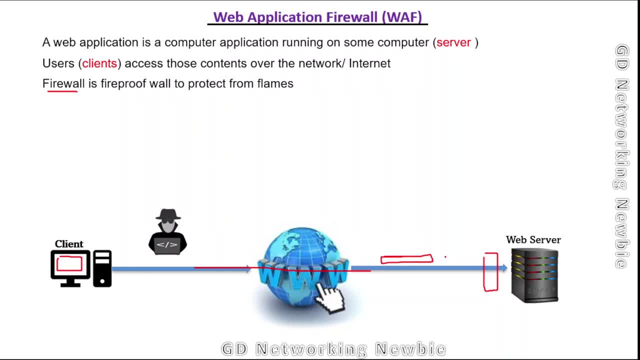 our network. it should decide that if a packet is arriving or if a packet is trying to reach on this side, then whether that packet should be allowed or that particular packet should be discarded, so that should be dropped out. so in that case this firewall needs some decision mechanism. 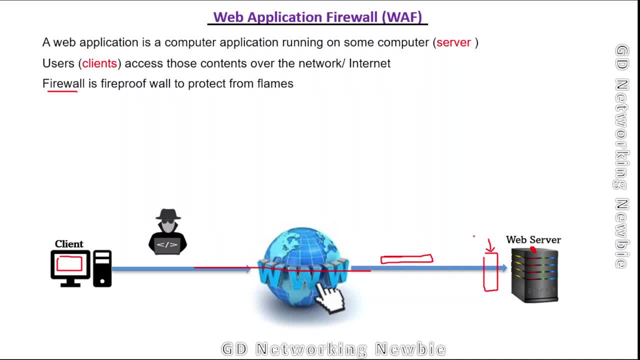 and how to make decision, or this needs some training or some pattern. so for that, this firewall works in use on the basis of different techniques, or those techniques can be like. they can decide on the basis of source or destination address. it means if a packet arrives here at the firewall, so firewall can look at the ip address. 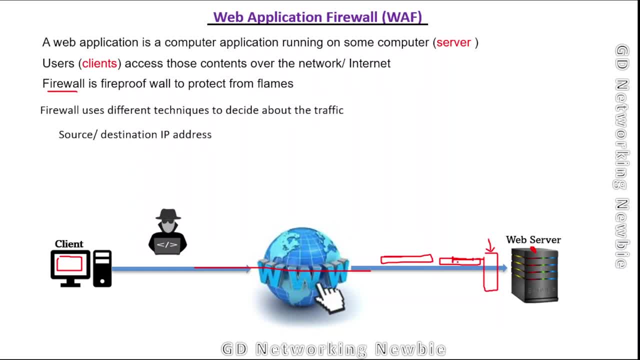 let's say source ip address or the destination ip address, and let's say in the source ip address: if firewall sees that this packet is coming from some network which is not reliable, so in that case this firewall can drop that packet. maybe that that firewall need not allow that packet to reach on this side. 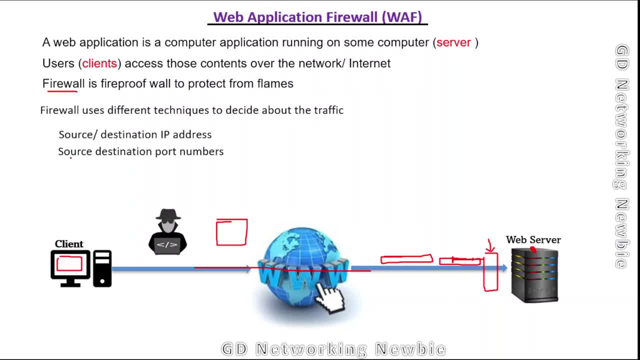 or the firewall can also make decision on the basis of, let's say, source or the destination port numbers, and the firewall can also make decision on the basis of some state or the record. record means that this packet isori is already registered and so that this package is possible to use. 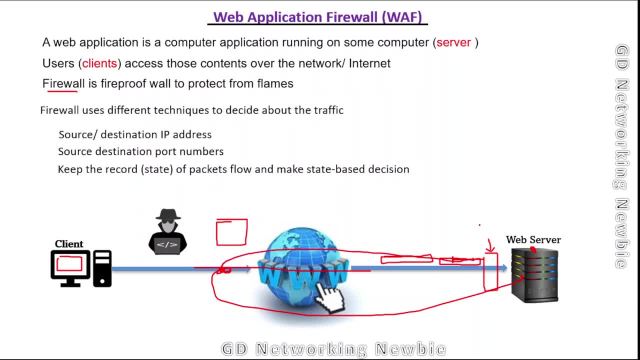 but the other way that this packet is already registered is a particular machine where this packet is still in the same particular location. this is what we want: this machine is in the same location or place, and then we want to allow that this packet to be able to reach on this side. 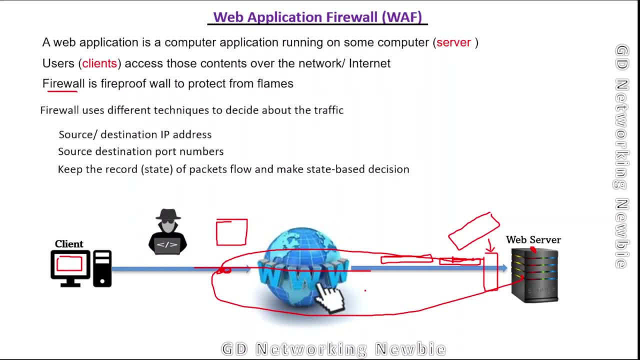 of the platform. so in this case time, some request for some machine or some machine has sent some request to some other machine and, as a result of that request, there may be some traffic coming back. web application firewalls and these web application firewalls are designed specifically to protect our web application, and this is done by 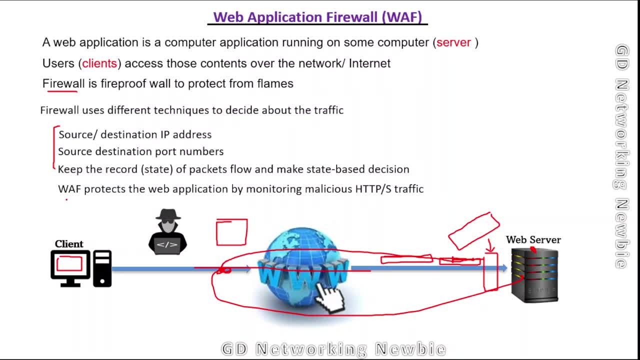 monitoring in general by monitoring the malicious HTTP or HTTPS traffic. and now, if we look at the layers, then these firewalls which mostly work at layer 3 and layer 4, so let's say on layer network layer and the transport layer. so these types of firewall are called Network firewall and the web. 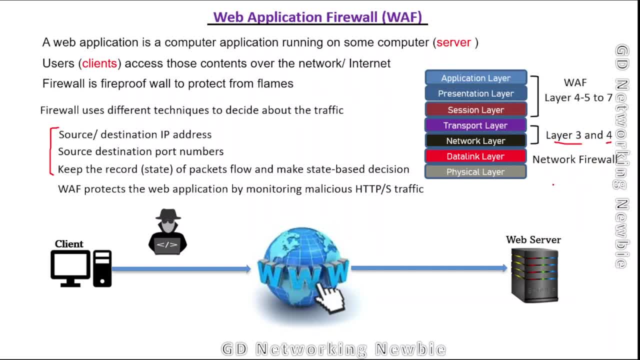 application firewalls are the firewalls which generally operate at layer 4, 5 to 7 aspect layer to the application layer. so in general, I mean this is rough idea. so this web- they work on these layers and their principal or the prime job is to secure our web applications from. 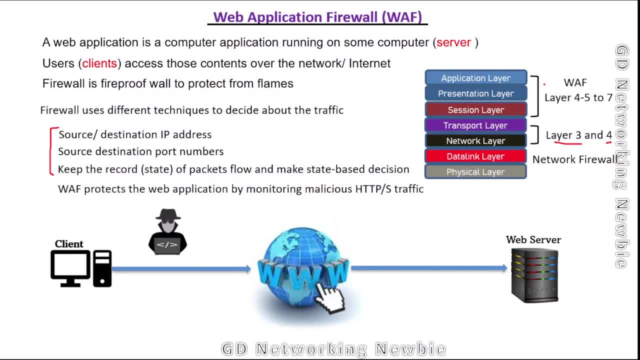 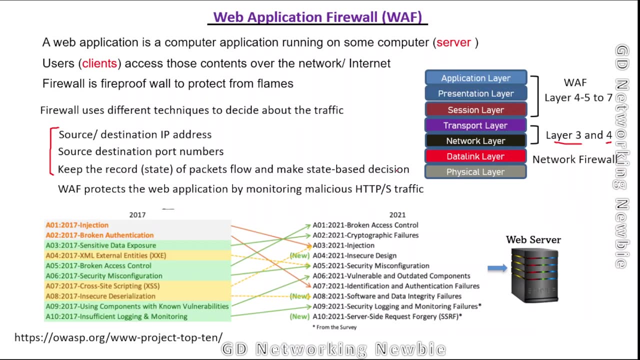 from different attacks. Our web application can have different weaknesses or vulnerability which have- I mean which we can find- those commonly known vulnerability on the website, which is maintained by Open Web Application Security Project. You can see this here. This is the website and on that website, 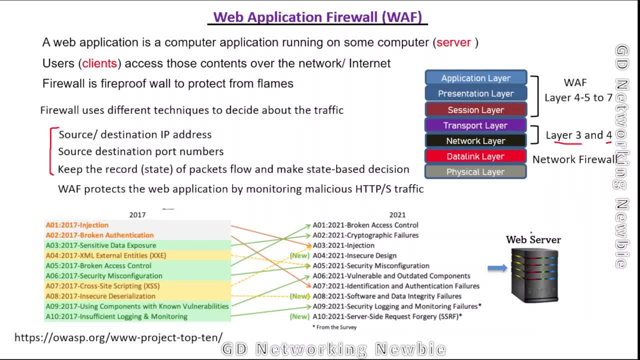 we can find the common vulnerabilities which are found in web applications- And this is actually list of top 10 vulnerabilities which are generally found in web application. So these weaknesses can be broken: access control, cryptographic failure, injection, insecure design, security misconfigurations. 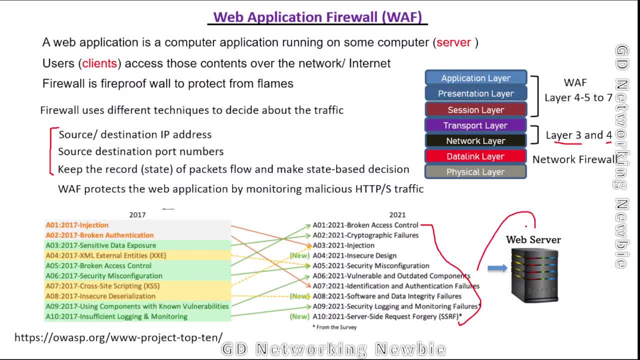 So these all vulnerabilities can be in our particular web application, and to secure our web application we need some firewall, and those firewalls are known as web application firewalls or the WEF, And I'll also put a link of a very useful document. 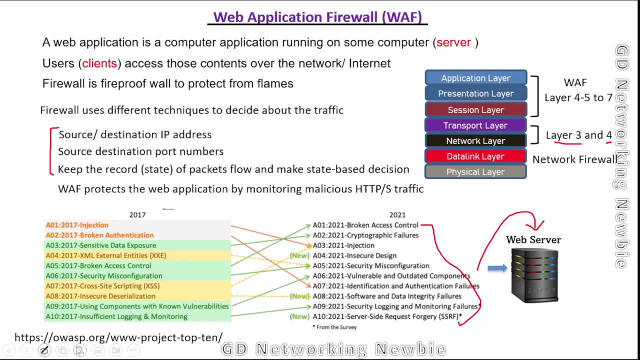 which is this There on this website so you can find the description in the description section, the link to that document. that will be very much helpful that what kind of products are available in the market which we can use as a WEF. 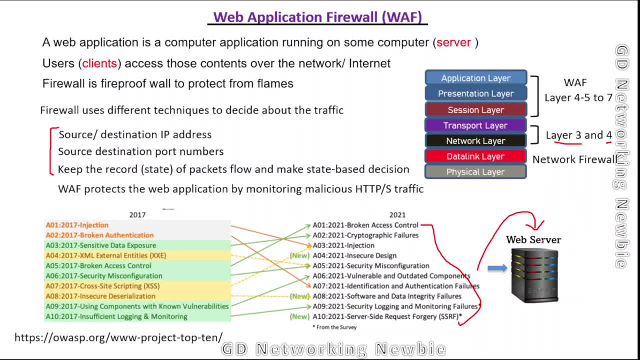 because there are different vendors which are selling out their products, And then how these different WEF or the web application firewall work. these different techniques are also discussed in that document And from that document maybe in our next video I'll discuss that- how we can detect these firewalls. 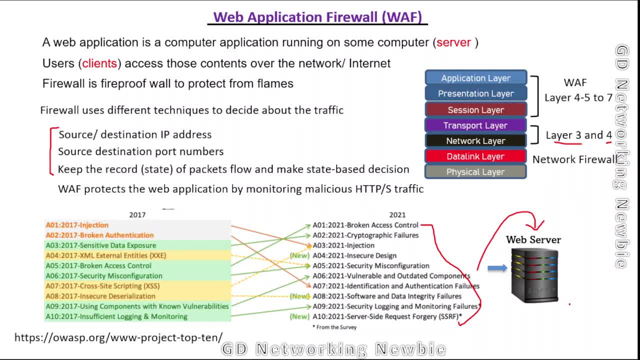 Because from ethical hacking point of view or from pen testing point of view, we should also be able to detect firewall if any web server or any server is using particular web application firewall. So if we have the information about, let's say, WEF, which is being used by our target machine. 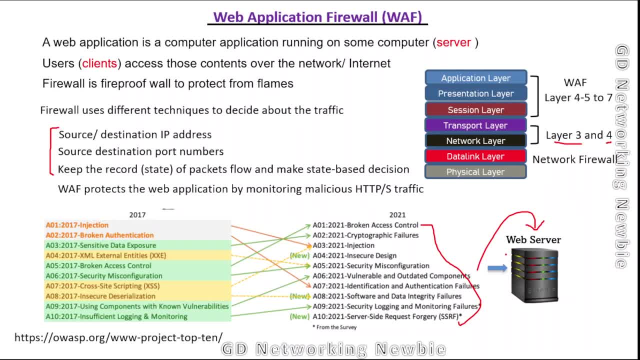 then maybe we can design some tools or tricks by which we can evade those firewalls and maybe we can attack it. So this is something maybe we'll see in our next video For this. this was a brief introduction about WEF. Hopefully for some of you this may be useful.